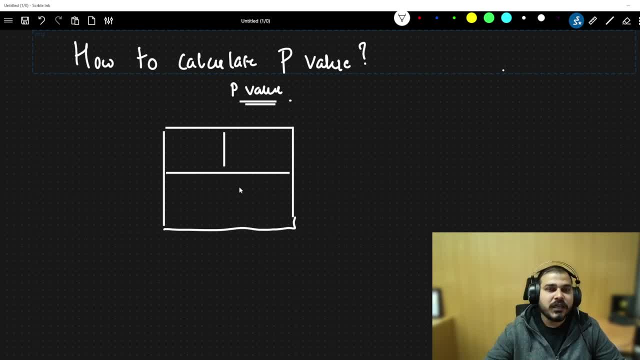 probably in this region. you know I'll be touching to basically move the cursor and all. So if I say, let's say that most of the time I'll be touching in the center region, so I can definitely draw a normal distribution curve kind of thing like this and suppose, if I say that at this point, 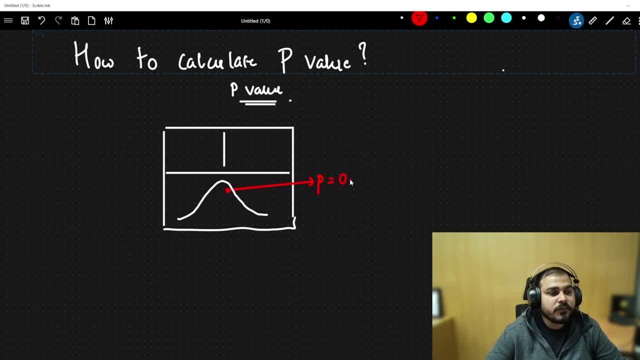 okay, my p-value is point eight, right? So this basically means that out of every hundred touches, out of every hundred touches okay in this region, I will be touching 80 times okay. So this is basically the probability of touches that I am going to do, okay. and similarly, if I probably touch in this region and suppose 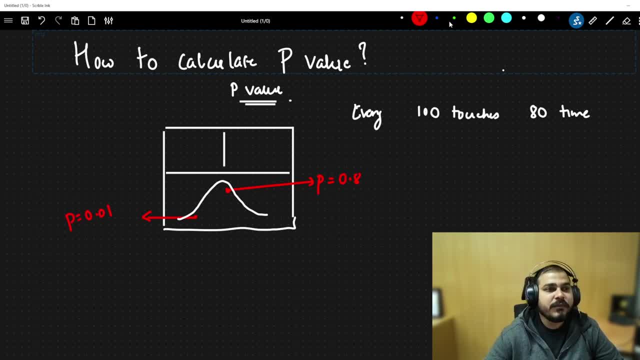 let's consider that the p-value is 0.01. this basically means that out of every hundred touches, that I am actually touching this point. So if I say that out of every hundred touches I will be touching in this particular mouse pad, I will be touching in this region one time, right? So this is. 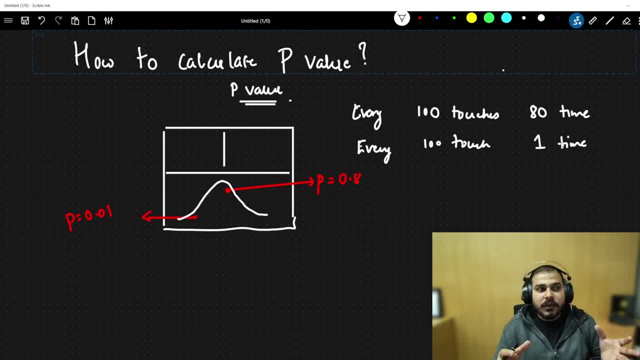 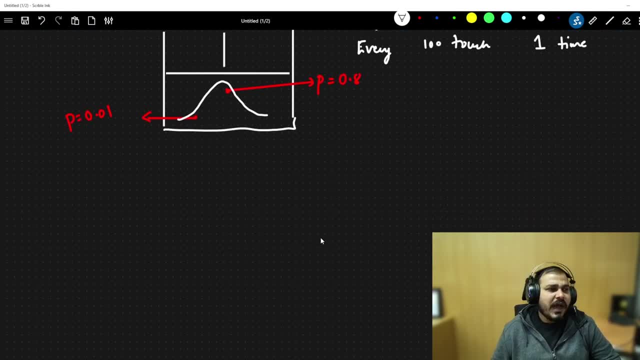 what basically p-value means. okay, Now let's let's solve a specific problem. okay, Now let's solve a specific problem, and this problem is basically called as z-test. Suppose I have a specific problem which I want to really perform with the help of hypothesis testing. okay, So let's consider. 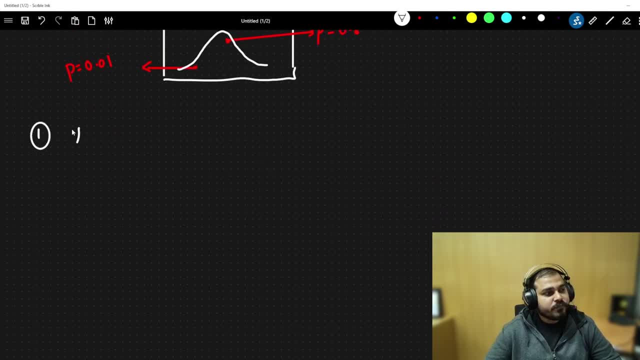 a problem statement. Now, in this problem statement, let's say that the average, the average weight of the average weight of CTA is, let's say that it is 72 kgs. okay, So this is my question: 72 kg with a standard deviation, with a standard deviation of value 4. okay, So this is the standard deviation. 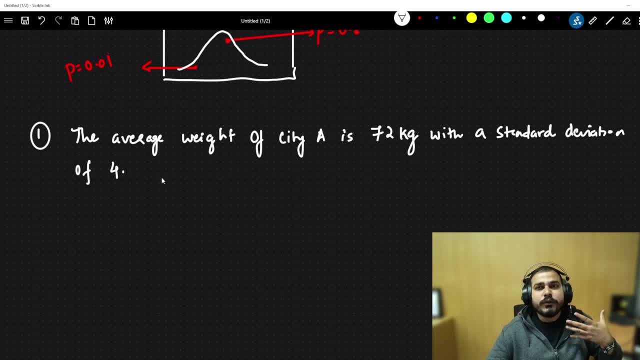 I feel that I don't believe it. so I really want to do the test and try to find out. I really want to check out whether this is actually true or not. So you know whether this mean, this mean, you know the average weight or this mean is true or not. So what I do is that I pick up a sample, a sample. 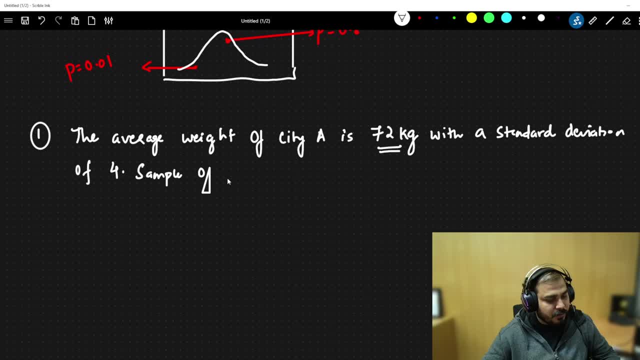 of, let's say that a sample of 36 people has been picked from the city has been picked, and And when I calculated the mean, where the mean was, let's say, 74,, okay, So the mean was 74. I need to see that, whether this true mean is different or not. 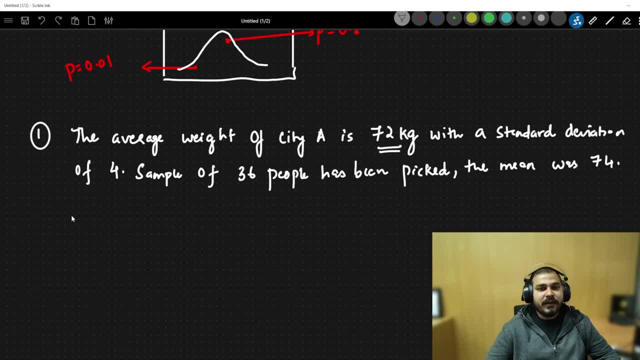 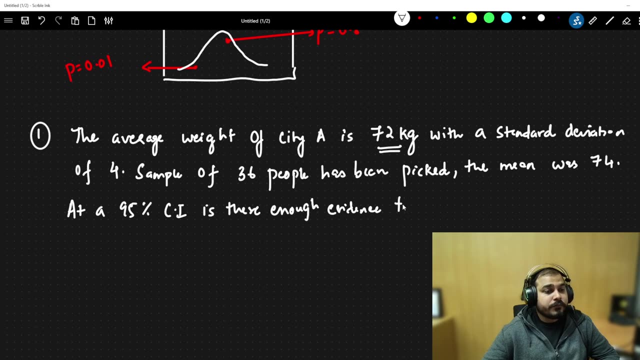 This is the exact question. So here I will basically saying that at a 95% confidence interval- suppose I am considering 95% confidence interval- well, is there enough evidence to support null hypothesis? Now you may be considering: what exactly is null hypothesis over here? 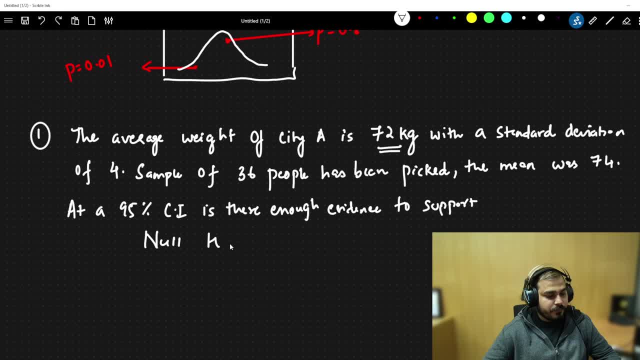 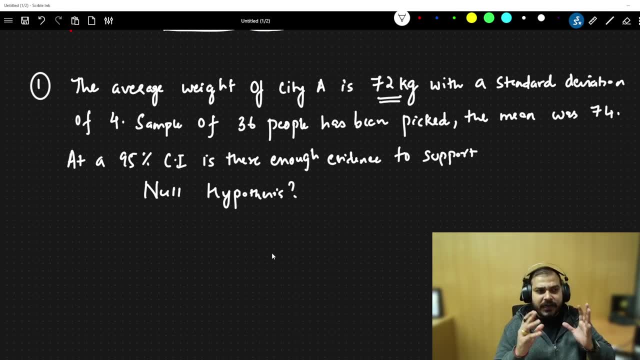 I will discuss about it- To support null hypothesis. So this is my question over here. okay, So what is the problem? statement: I understand that the average weight of people in a city, I should say of people in city A, is 72 kg, with a standard deviation of 4.. 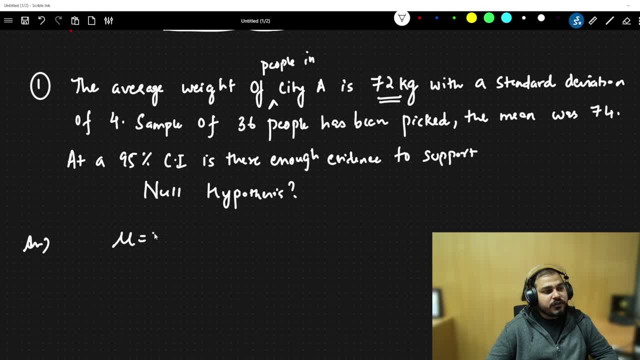 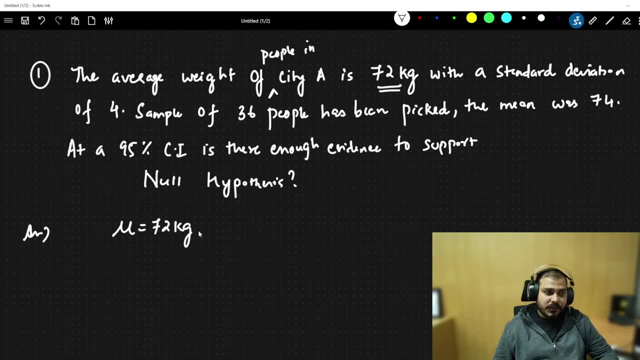 So, first of all, let's see what all information is given. Your mean value is basically given. I have already uploaded videos on how to calculate or how to perform different types of hypothesis testing. This: what kind of hypothesis testing I will be performing. I will talk about it. 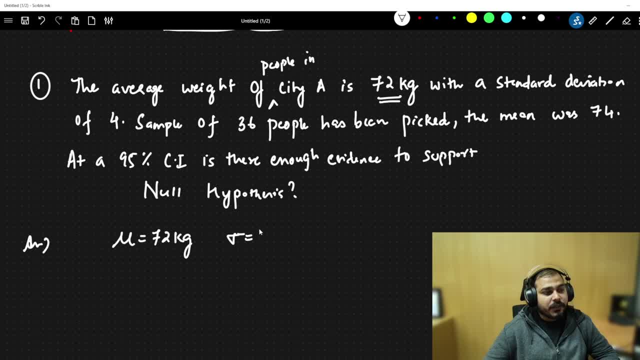 Suppose the mean is 72 kg Over. here the standard deviation, the population standard deviation, is 4.. The n value sample of 36 people has been picked and then the n value sample of 36 people has been picked. So the x bar, that is the mean of those sample, is 74.. 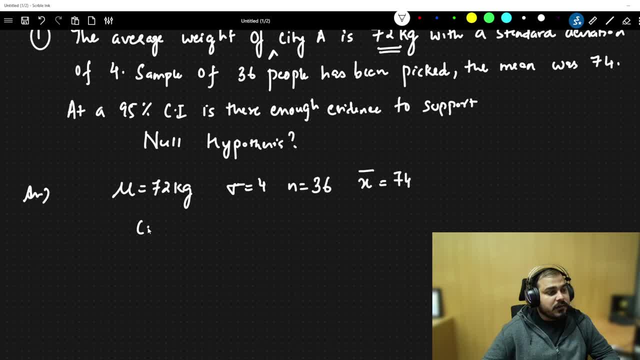 So this all information basically I have. And here the information of confidence interval is also given. That is 95 percentage. Okay, Whenever we have confidence interval, with the help of this we can definitely be able to calculate our significance value. 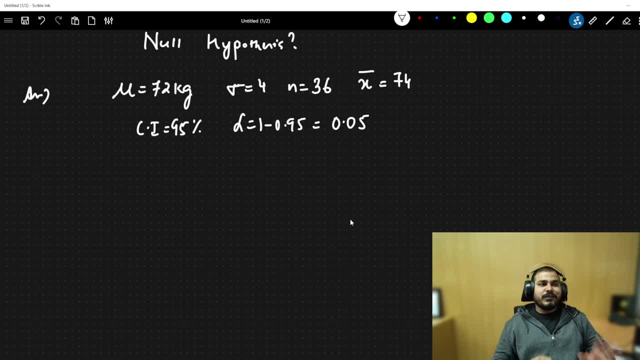 So here our significance value is 0.5.. Now remember, guys, we can solve this problem with the help of hypothesis testing in two ways. One is directly: calculate your z score, And probably do it, The reason why I will be using over here z test. 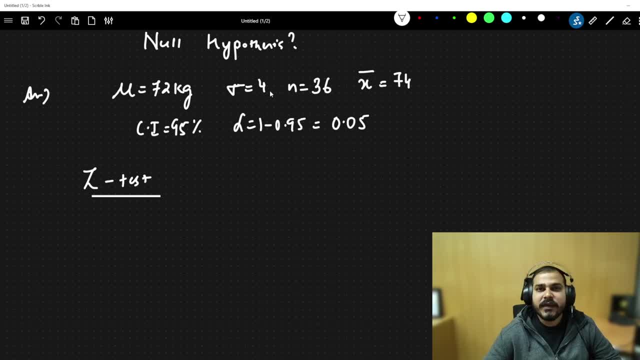 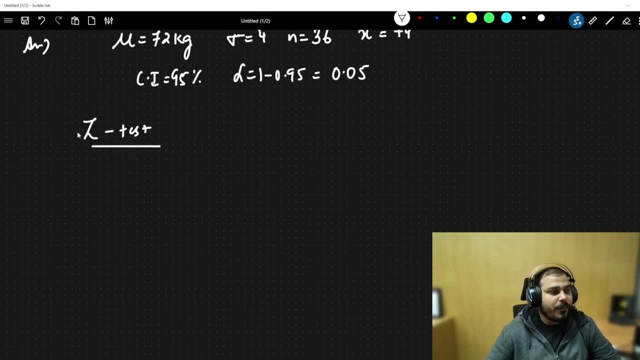 Because, understand, in z test the population standard deviation will be given And apart from that, your sample size will be greater than or equal to 30.. Okay, So both the condition it is basically satisfied. So my first step will be that define my null hypothesis. 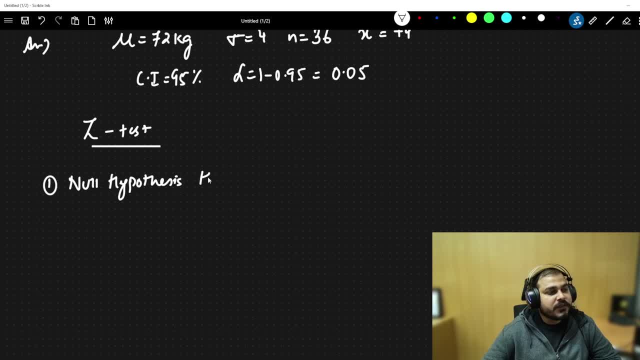 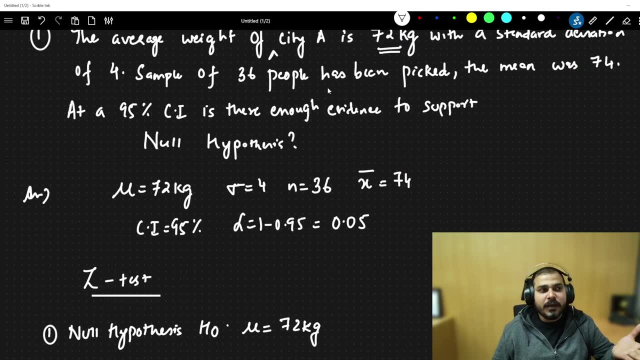 Now my null hypothesis over here basically says that which is specified by x0,, your mean is equal to 72 kg. That is what I am actually trying, So I am going to test by picking up a sample of 36 people. 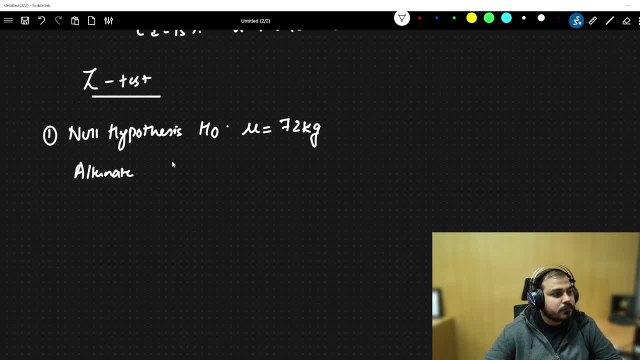 Right, Then your alternate hypothesis, Then your alternate hypothesis will be h1,, which will not mean will not be equal to 72 kg. Right? If this is rejected, obviously, that basically means that it is not equal to 72.. 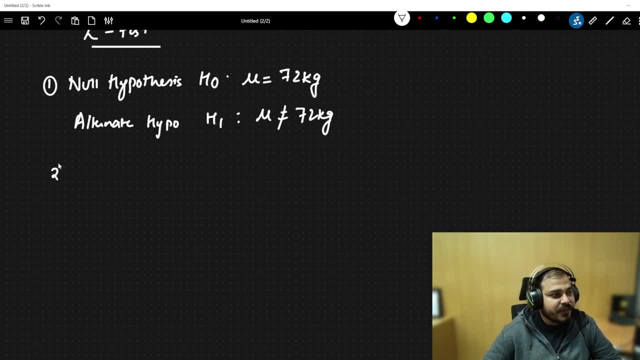 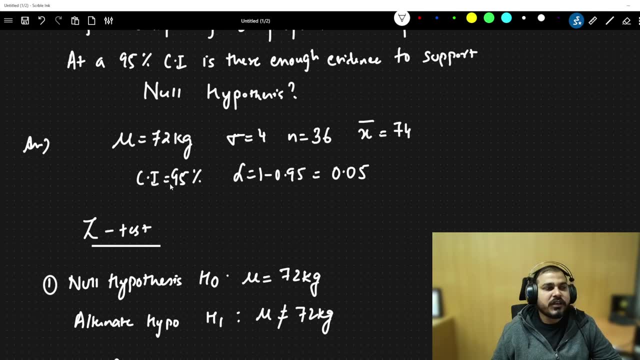 Okay, Now understand the second step. I will definitely talk about my significance value, which is nothing but 0.05.. Okay, So significance value is also given because I have. I was able to find it out from the confidence interval. 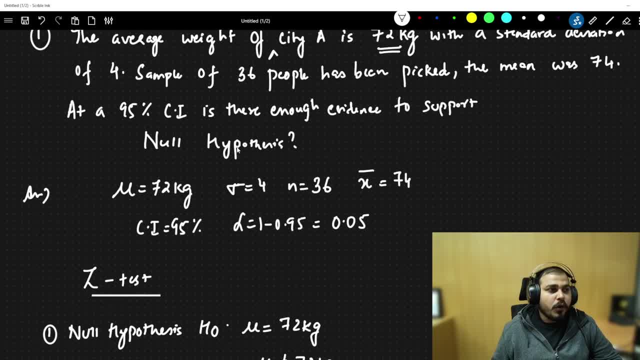 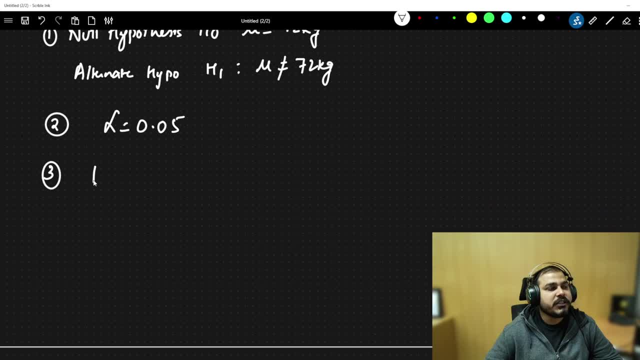 Okay, Now coming to the next step, which is quite important. Over here, you will be able to see that what test you need to apply, you have already got it Right Here. we will basically define our decision rule. 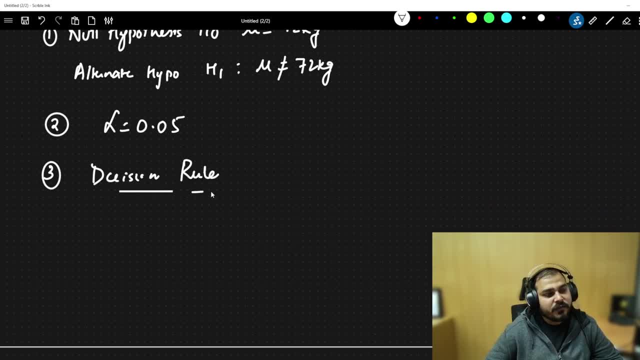 What should be our decision rule Now in this particular case? my decision rule now: first of all, you need to find out whether it is a one-tail or two-tail test. Now people also get confused. How to determine whether it is a one-tail or two-tail test? 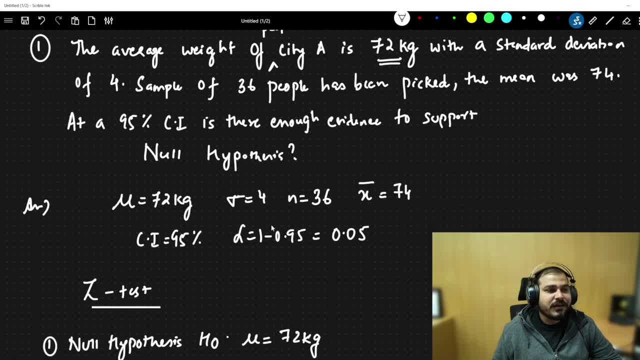 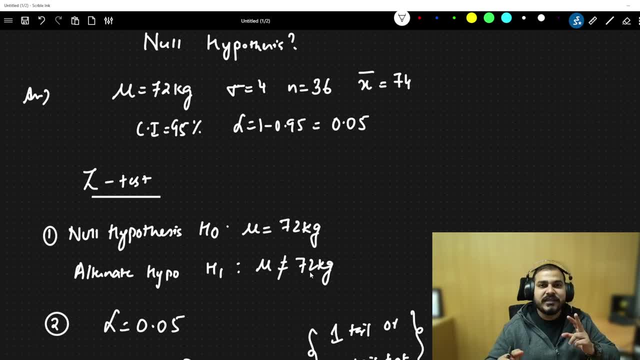 Because, understand, we are basically checking whether the mean is 72 or not. It can be greater than 72,. it can also be less than 72, right? So in this particular scenario, both are there. right, Because we are checking whether mean is equal to 72. 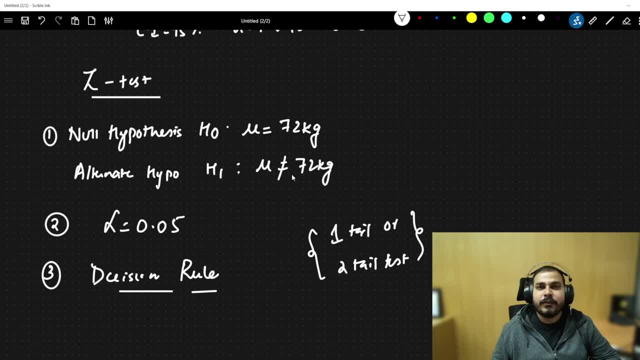 or mean is not equal to 72. If we go to the alternate hypothesis, even though the mean is less than 72, it basically means the mean is not equal to 72. If it is greater than 72, that also means the same thing. 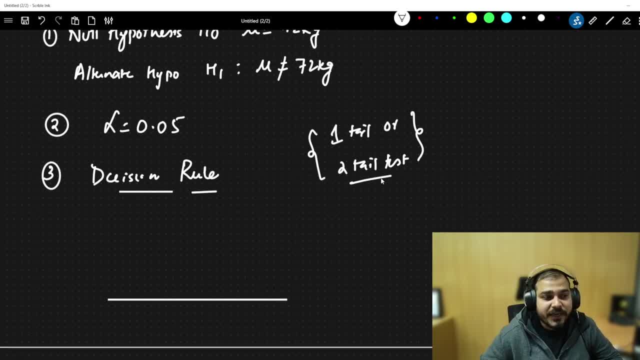 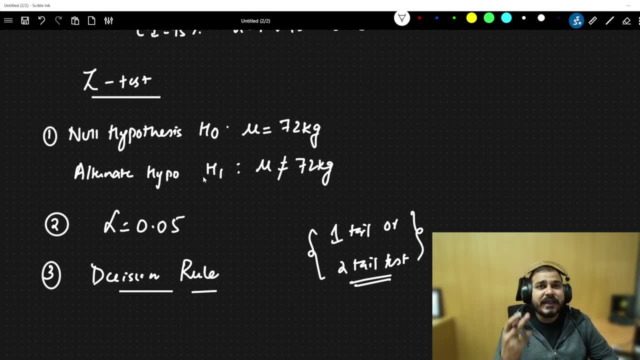 that it is not equal to 72.. So in this particular case, we will definitely be applying two-tail test. If the condition was that check whether the mean is greater than 72, at that point of time we can use one-tail test. 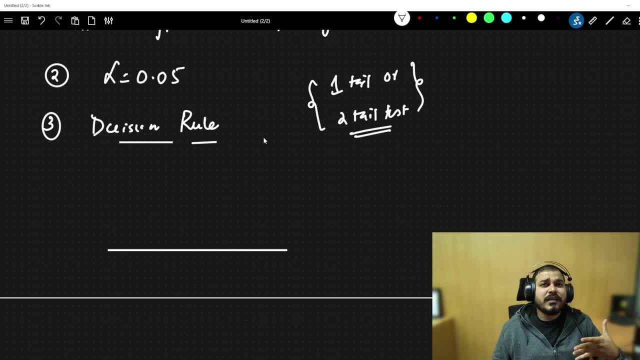 But here my scenario is to check from the sample whether the mean is not equal to 72.. It can be greater, it can be lesser. So while specifying the decision rule, always understand over here in a two-tail test. 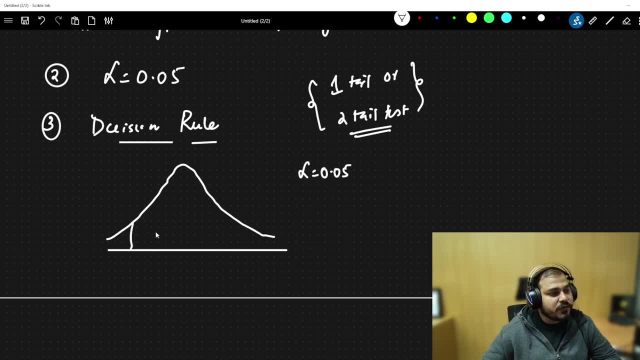 based on our alpha value 0.05, we will be using two-tail test. Now, in two-tail test, always understand this will be our 95% confidence interval. the remaining is 0.05.. So here you will be getting 0.025.. 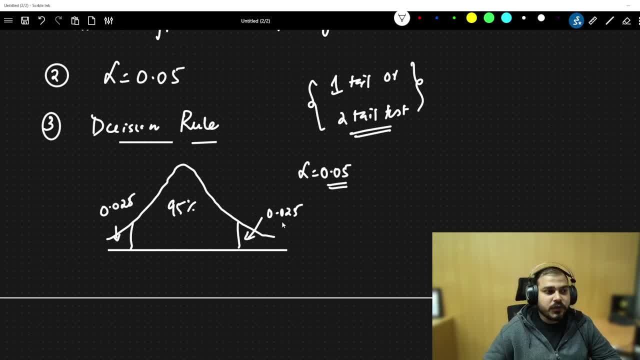 Here also, you will be getting 0.025.. Okay, So here are your two values with respect to this. Okay, Because this gets divided. These both are symmetrical. right, Left and right region are symmetrical. Now you need to understand what kind of test you are going to use. 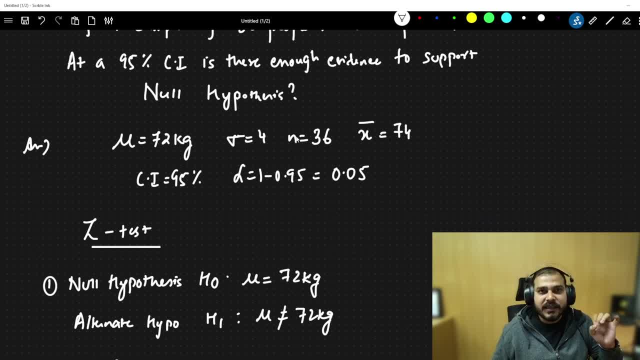 As I said, that population standard deviation is given and n value is greater than 36.. So the statistics that we are going to use, So the statistics that we are going to use, So the statistics that we are going to use. 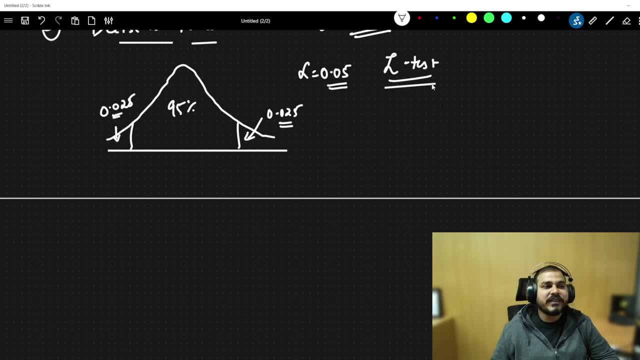 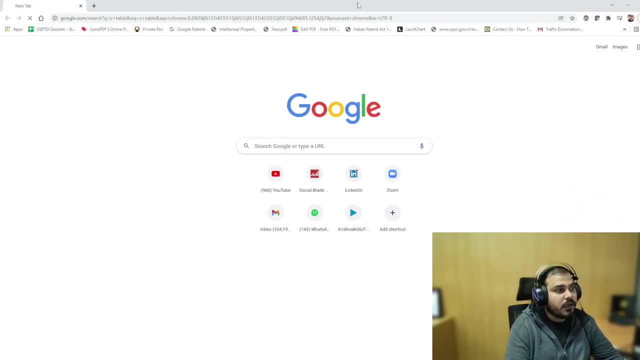 is something called as Z-test. Now, how do you find out Z-test? The Z-test is very much simple. I will open a browser Here. I will basically open a Z-table first of all Because I need to know right. 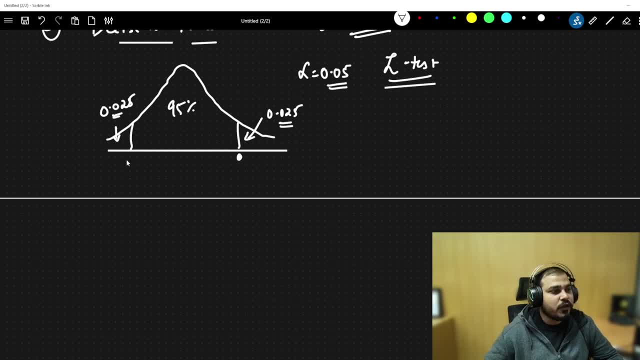 What is this value? What is this specific value of 0.025?? And what is this specific value of 0.025?? What is the area under the curve Right? I need to understand. what is this entire area under the curve? 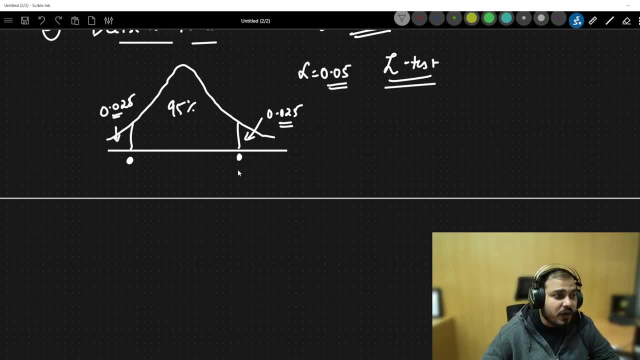 Okay, And based on this, what should be the Z-score of this value, What should be the Z-score of here And what should be the Z-score over here? Okay, I need to find it out, this, And in order to find it out, what I will do is that. 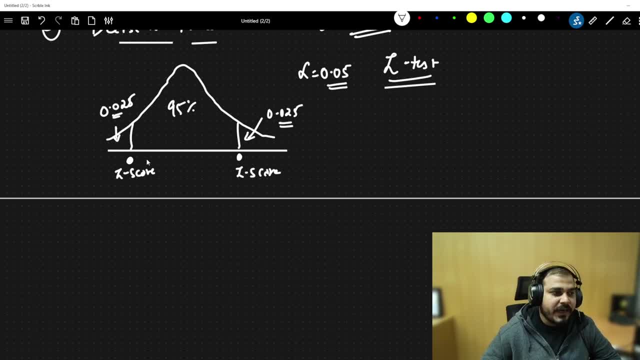 let's compute of this side. first of all. If I compute of this side over here, only the negation will be there right Over here. if I am getting a positive value, this will be the same negative value, Okay. 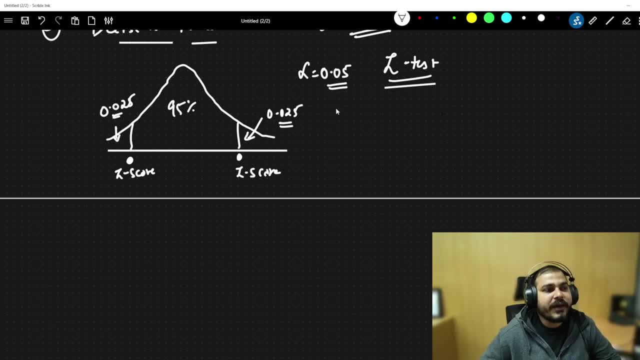 Because both are symmetrical, Right? So in order to calculate now, first step, I need to basically take up this 0.025 and subtract with the entire area, Because, see, the entire area is 1.. Okay, And then I subtract with this. 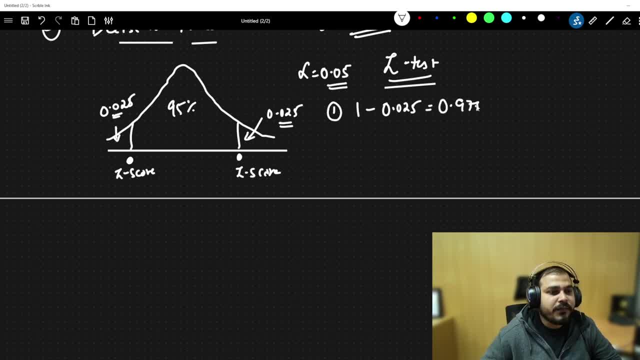 That basically means this is nothing but 0.9750.. So this entire area is 0.9750.. I need to find out the area of the curve, Right Area of the body. Here I can also write area of the curve or area of the body. 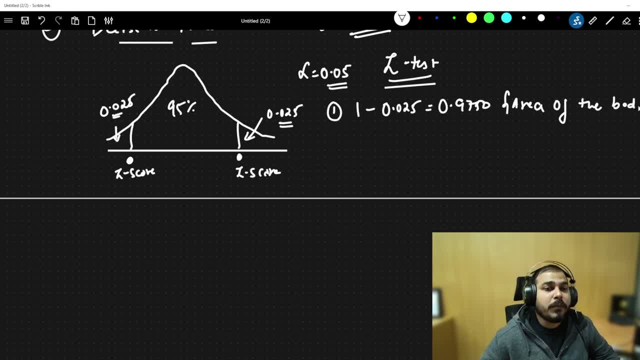 So here I am actually specifically trying to find out area of the body skipping this tail region. Okay, Skipping this tail region. So obviously I will subtract with 1 minus 0.025, which is 0.9750.. 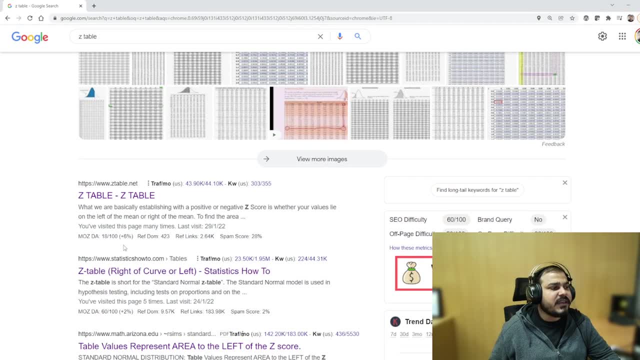 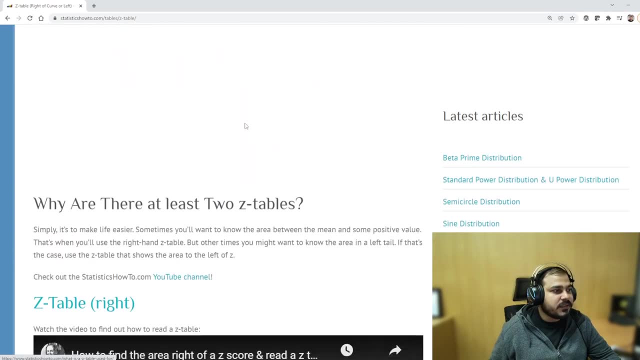 Now, if I go back, if I go back in the Z table, let's say that this is my Z table Here. you will be able to see that. Okay, So this, this values. you can see this particular table. 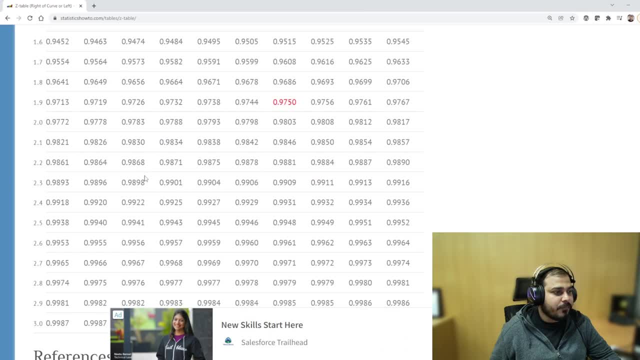 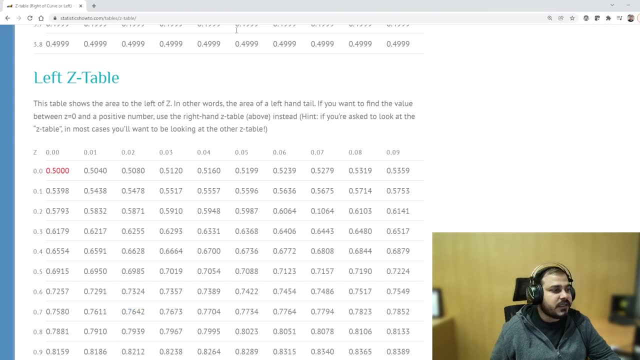 Okay. So when I say area under the curve, I am going to basically consider this table Right. So here is my table. Okay, So here is my table. I will just close this out. Okay Now, 0.9750.. 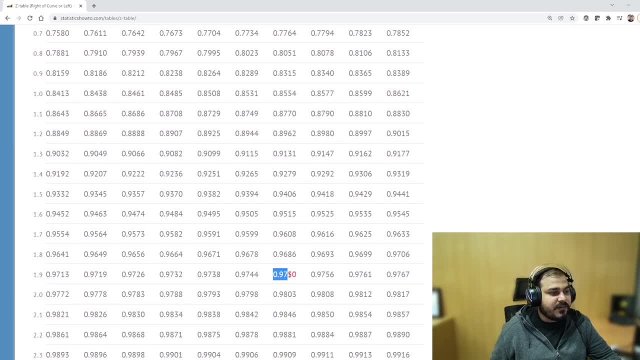 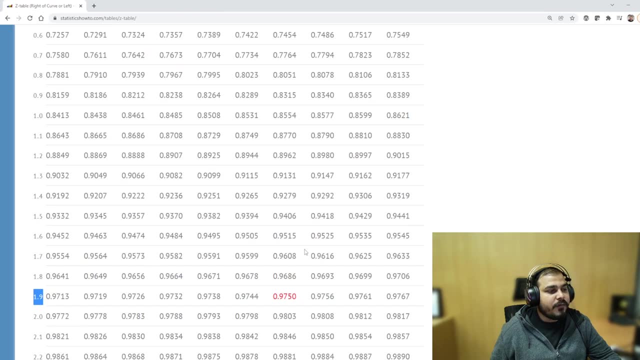 Just check where it is. So here you will be able to see 0.9750.. Okay, And based on this, what is the value? It is 1.9, 1.9.. And from this particular column, you will be seeing 0.06.. 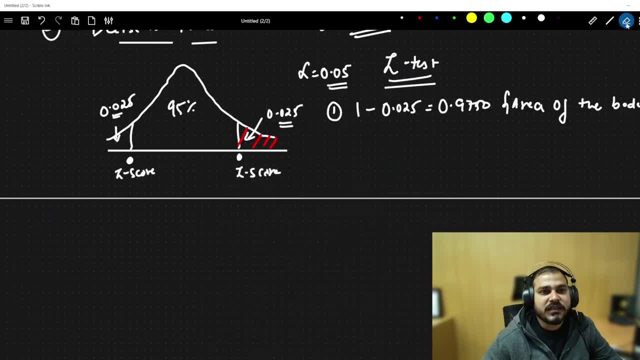 So it is nothing but 1.96.. So that basically means this Z-score value and this I have already explained in my previous videos. in statistics, This is plus 1.96 and this is minus 1.96.. Right. 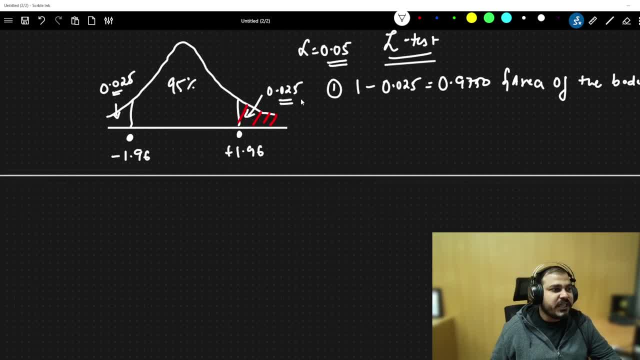 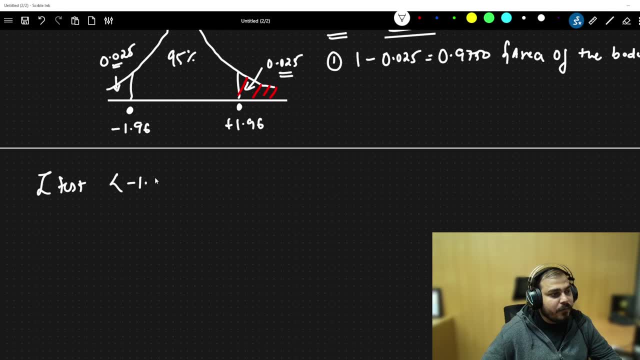 Minus 1.96.. So that basically means my decision will be that after I perform a Z-test based on the data, if it is less than 1.96 or greater than 1.96, I have to reject the null hypothesis. 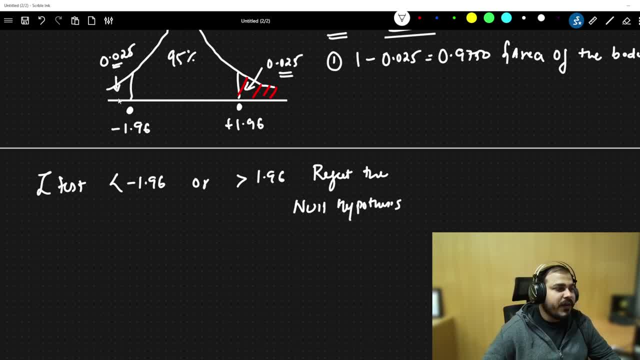 Okay, Because it does not fall in that confidence interval. If it falls in this region that is less than 1.96, I have to reject it. If it falls greater than 1.96, I have to reject it, Right. 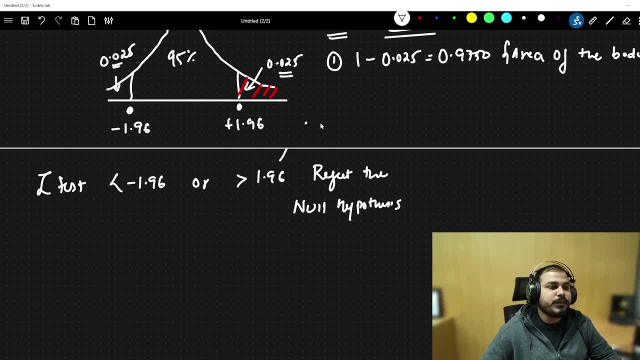 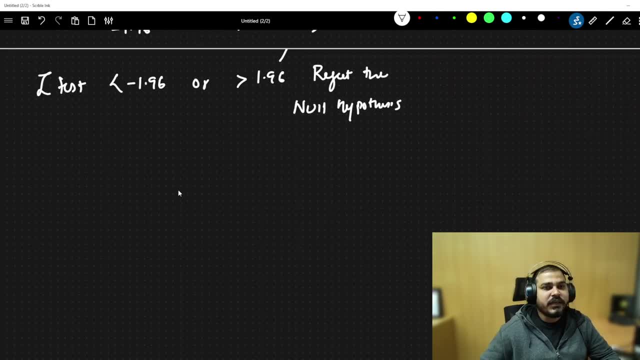 So I have written, OR So this is my decision. This is specifically my decision Right Now. let us go ahead and apply our Z-test, That is, our test statistic. So next step, what I am going to do, I will go and perform this. 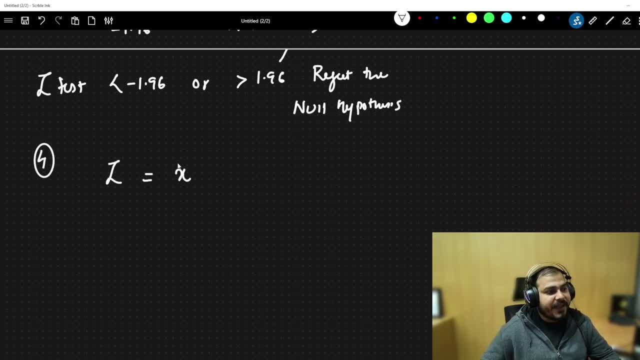 And for this, obviously you know what is the Z-score formula: X bar minus mu, divided by standard deviation, divided by root n. This is called a standard error. Okay. Sigma by root n. You can search for that also Okay. 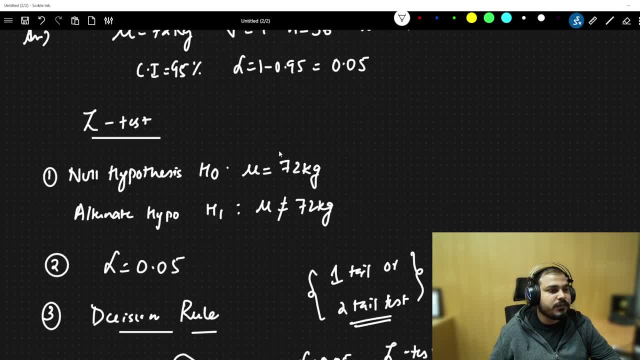 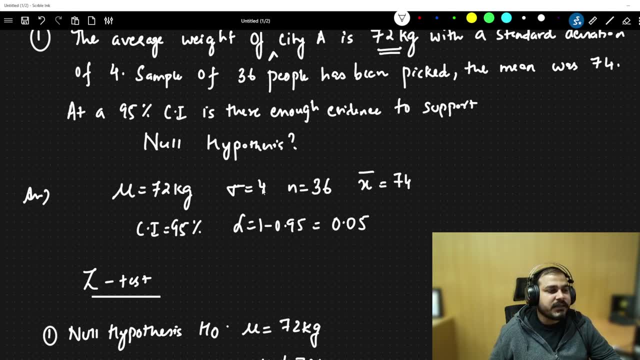 So what is X bar? X bar is nothing but what is X bar? If I see over here, X bar is nothing but 74.. Mu is 72.. Okay, And n is 36 and sigma is 4.. Right. 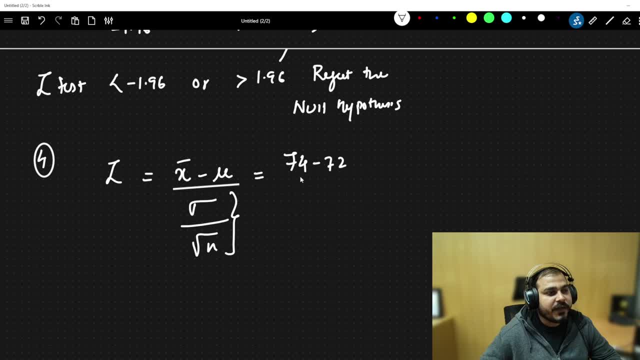 So what I am going to do? I am going to write 74 minus 72. Okay, Divided by 4, divided by root of 36.. This root of 36 will now become 2.. This 74 minus 72 is 2 divided by 4, multiplied by 6.. 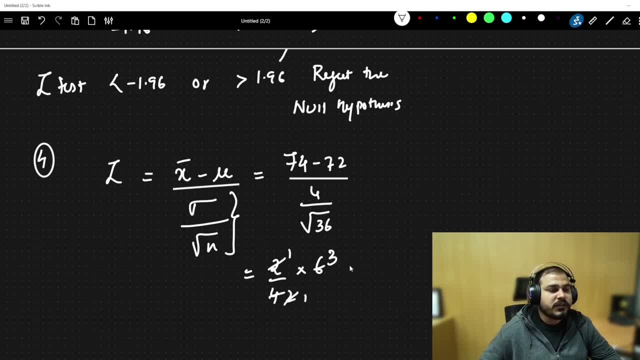 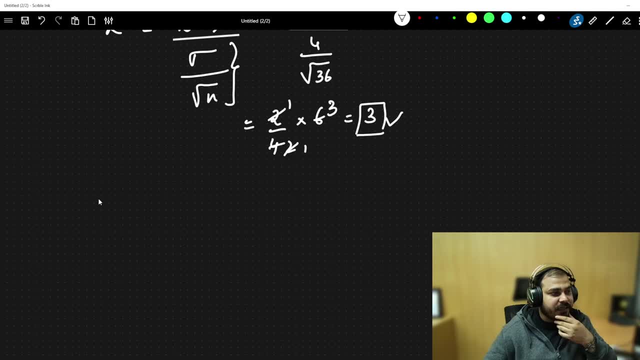 So 2 ones are 2, twos are 2, ones are 2, threes are. Now I am getting this 3 as Z-score, Okay, So what is the decision I can make? Definitely, 3 is greater than 1.96.. 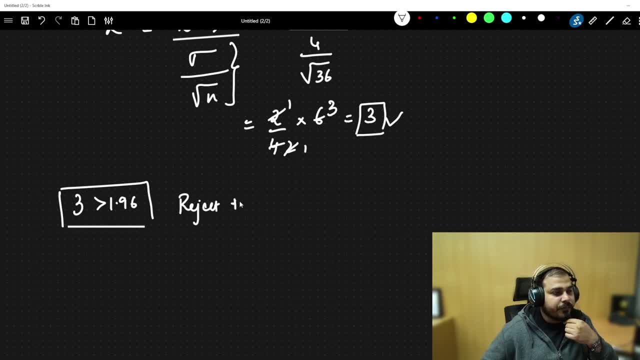 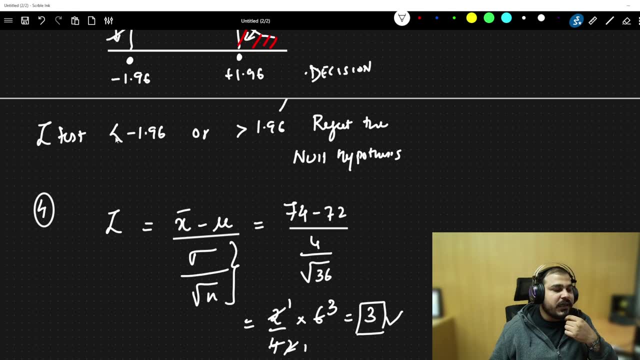 Okay, So we have to reject the null hypothesis. I told you right. we had two decision condition. One is if it is less than 1.96 minus 1.96, or if it is greater than 1.96.. 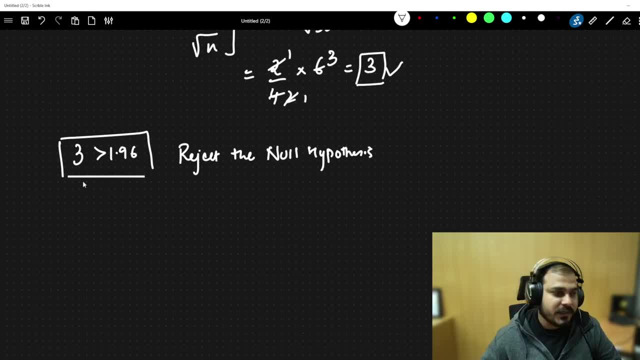 Now, in this particular case I have definitely got it is greater than 1.96.. Now, this way is the first way, by using significance value. Okay, By significance value, But when you do coding, when you do coding, probably you see something called as p-value. 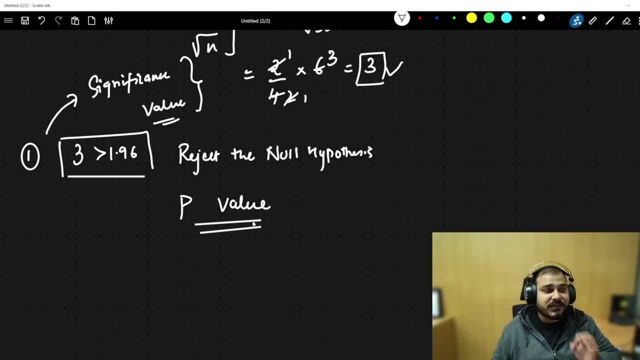 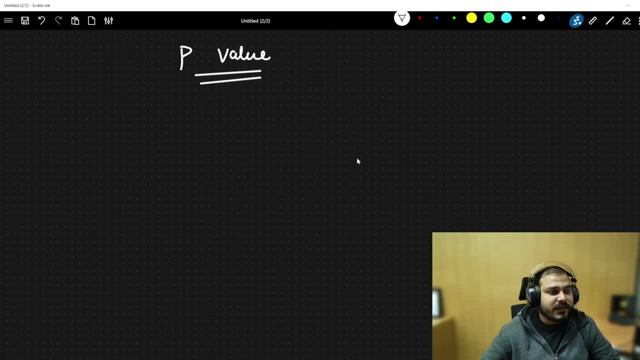 Now, what exactly is p-value and how p-value is computed? Understand this step. This is super important. Now I have got the Z-score. I have got the Z-score value as 3.. Right Now, let me do one thing. 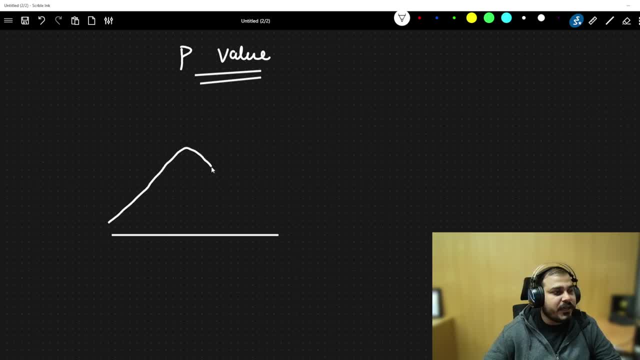 Let me draw the curve again. Okay, Now I am not interested in 1.96.. I am interested in 3.. So when I say 3,, so here will be minus 3,, here will be plus 3.. 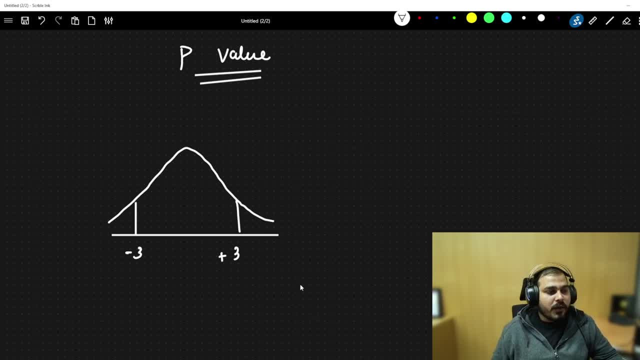 Right Now, again, I have to go to my Z-table and probably based on this 3,, what is the area of the curve that I should get? What is this area of the curve Or what is the area under this particular 95% interval? 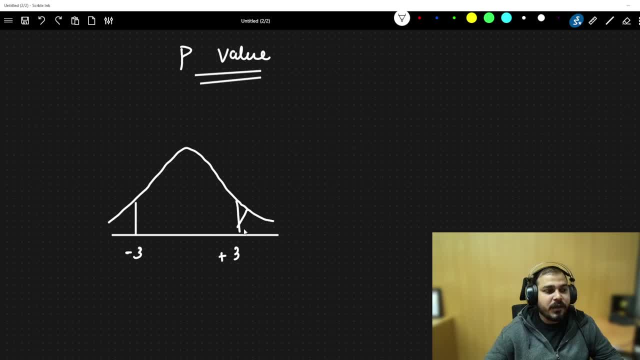 That we need to find out Now. see this Again. I am repeating you guys. See this: plus 3 is the Z-score that I got with respect to this, So I have written plus 3 and minus 3 over here. 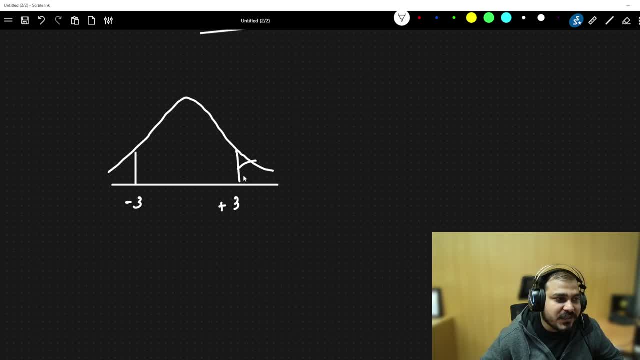 Now I need to find out this curve area. and how do I find out this curve area? It is very simple: I will just go to the Z-table and I will go to this Z-score and, based on this Z-score, it will give me the area under the curve, this entire area under the curve. it will give me. 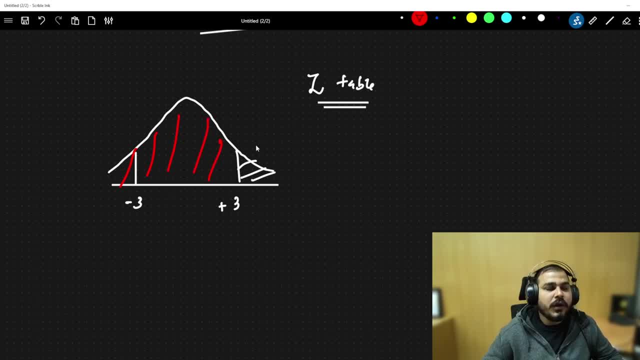 Right. So with that help, I will be able to find out. and now, in order to find out this curve, what I will do, I will subtract with 1.. Okay, I will subtract with 1.. That's it. 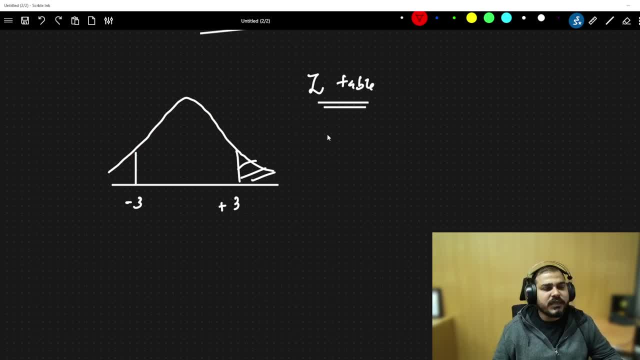 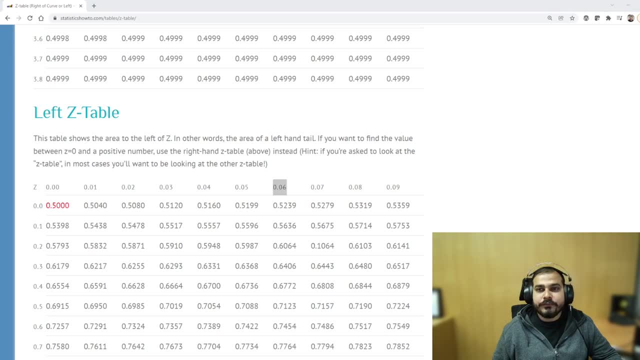 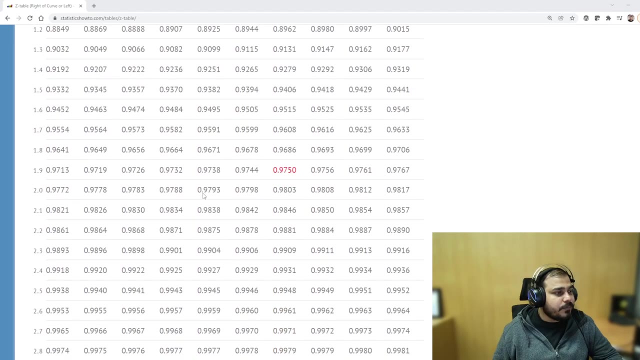 That is what I am actually trying to do, So let's see this. Okay, So I am going to remove this. I am going to go to my Z-table. Okay, I am going to go to my Z-table. Now, with respect to this Z-table, what I am actually going to do is that I will go and see where does 3 fall? 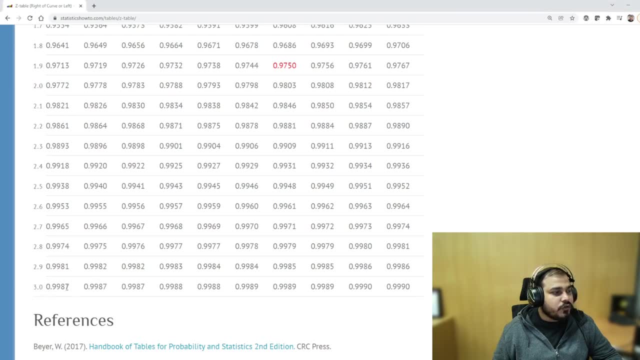 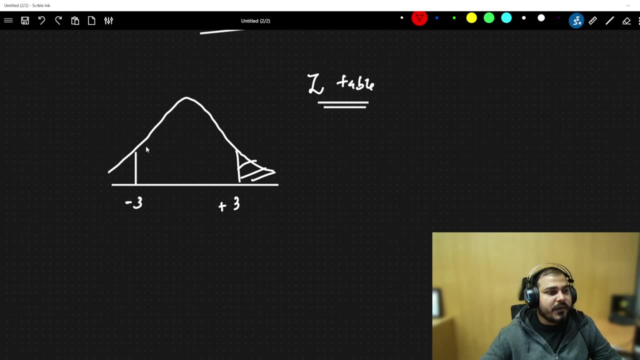 So here you can see, 3 is falling over here and I have got 3.0.. So this is my value: 0.9987.. Right, 0.9987.. So what I am actually going to do over here, I know, with respect to this, my area is nothing but 0.9887.. 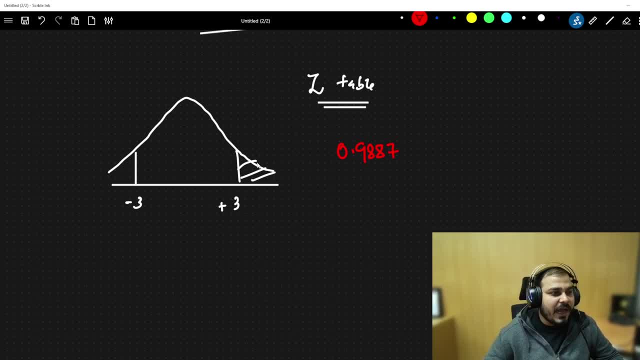 This is the area under the curve, Right Area under the curve. Now, how much should the curve belong here? and belong here Like I need to find out the area under this Right. So what I will do? I will subtract by 1 minus 0.9887.. 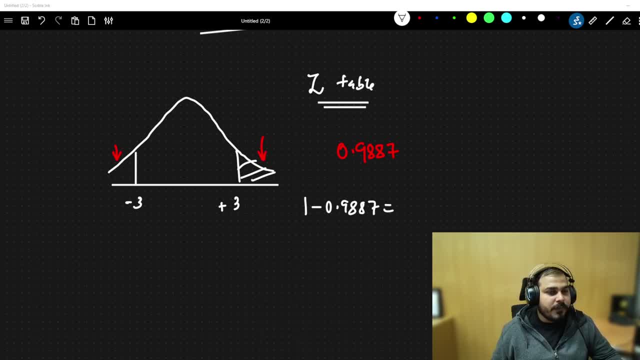 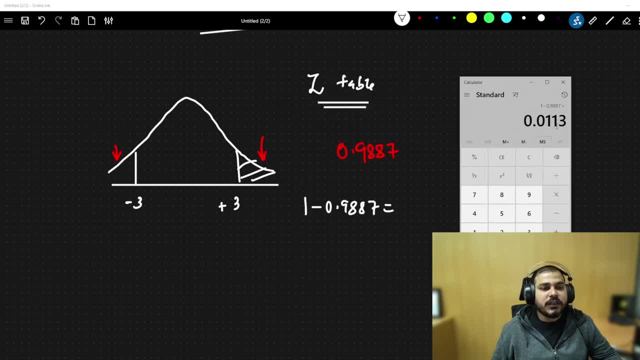 0.9887.. So I am basically getting 0.0113.. So here I will be getting 0.0113.. But understand, since this is a two-tailed test, I have one tail over here, one tail over here. 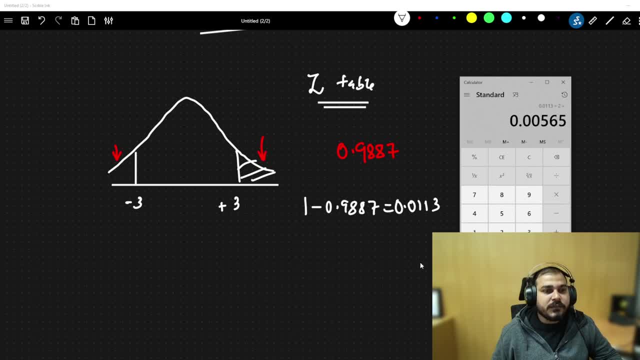 So this should be equally divided. So if I divide by 2, that basically means I will be getting 0.005.. Okay, So let me see again 0.00565.. So 0.00565 will be here. 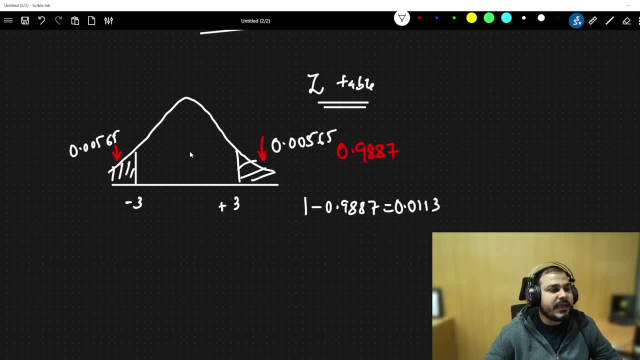 0.00565 will be there and remaining area will be present over here. If I add 3,, I will be getting it as 1.. So this 0.9887 will be present in this region, Right? So if I add it up, I will definitely be getting 1.. 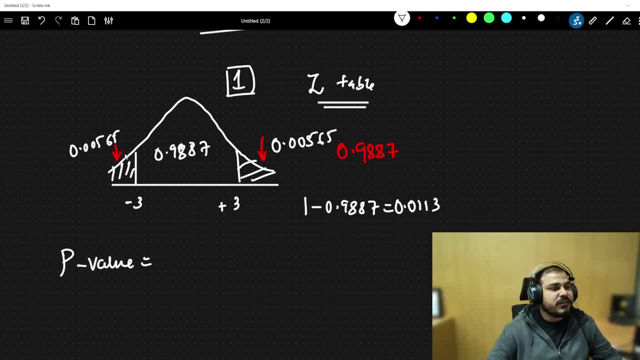 But still we did not understand what is p-value. So p-value is nothing but this area plus this area. So if I add 0.00565 plus 0.00565, I am actually going to get 0.00565.. 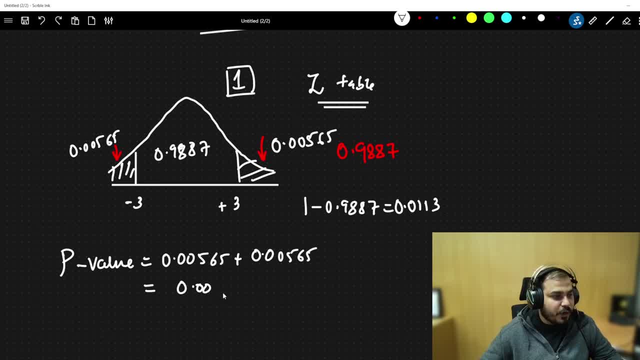 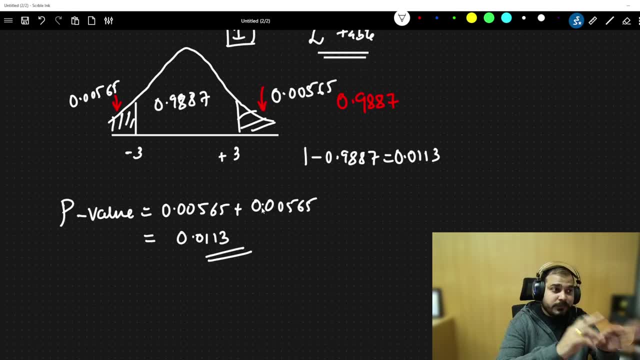 So I will get 0.00113.. Right, So 0.0113.. Now, once I get it, I hope the calculation is right. but focus on the things that I am actually doing Now: how p-value is related with significance value, because this is how encoding also will do. 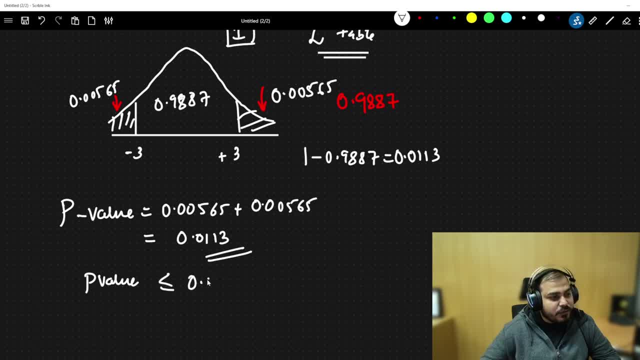 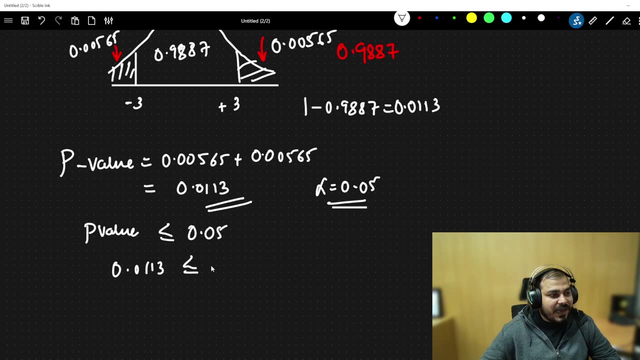 Now this is my p-value. We have to check whether this is greater than or equal to 0.05, which is my significance value. My significance value is 0.05.. Right Now, you can definitely see that 0.0113, okay- is obviously less than or equal to 0.05.. 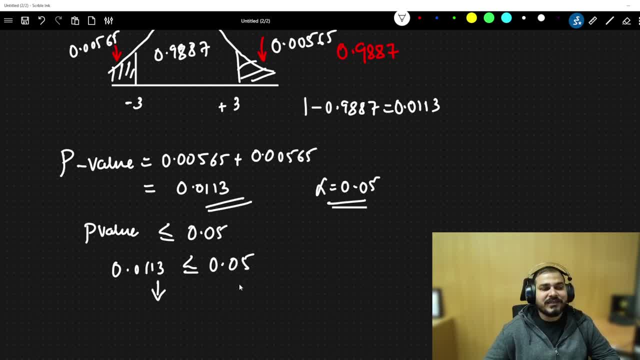 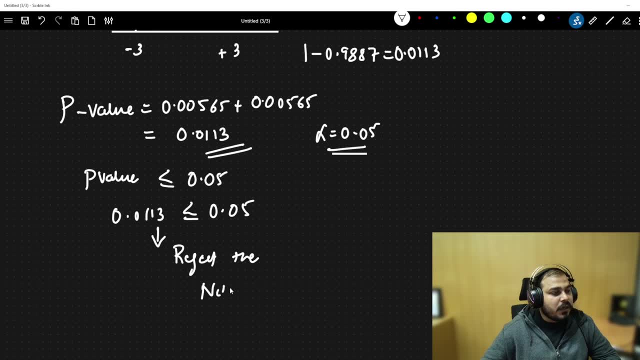 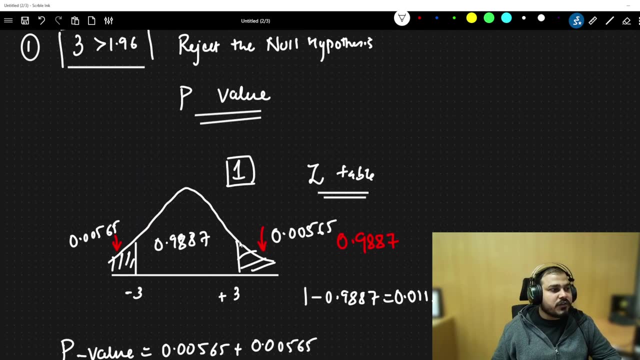 So what we do in this particular case: whenever the p-value is less than significance value, we reject the null hypothesis. Now see from both this scenario. we are getting the same answer Right From this scenario also. this is my second scenario. 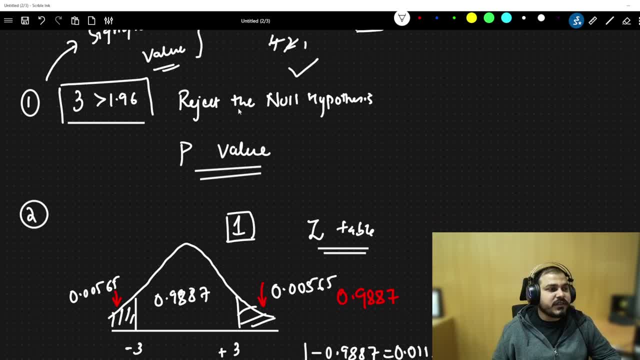 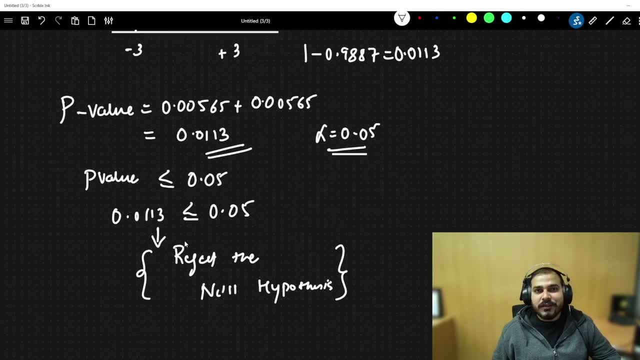 Which I am actually writing From this scenario. also, I am rejecting the null hypothesis. Here I am just focusing on the z-score and trying to find out based on the decision boundary. Here I am just trying to find out the p-value and then comparing whether to reject the null hypothesis or not. 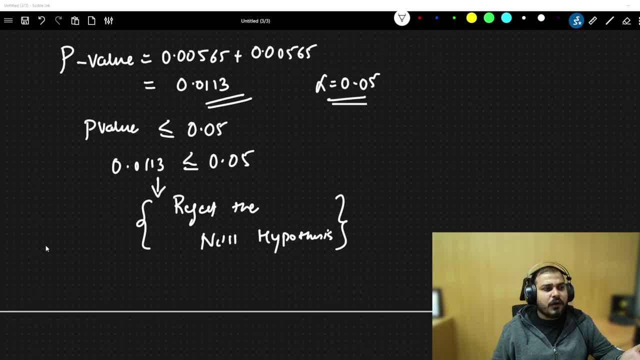 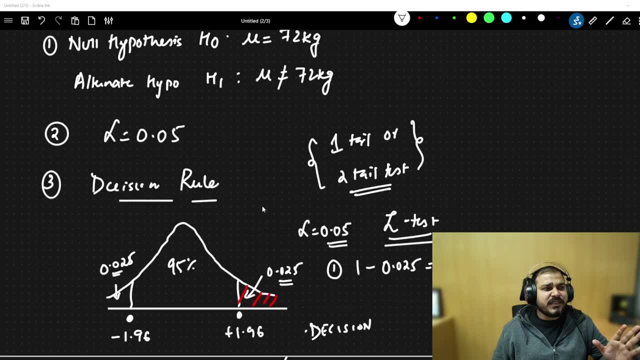 Right Now let me like. this is the step, And this is how simple a p-value is basically computed and whether it can be compared with this significance value: Very, very simple. See the steps In front of you. I have given an example. 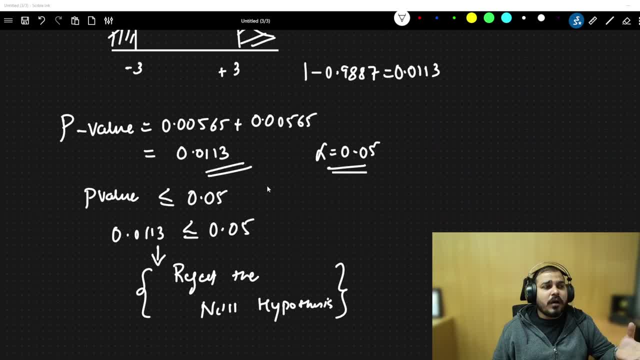 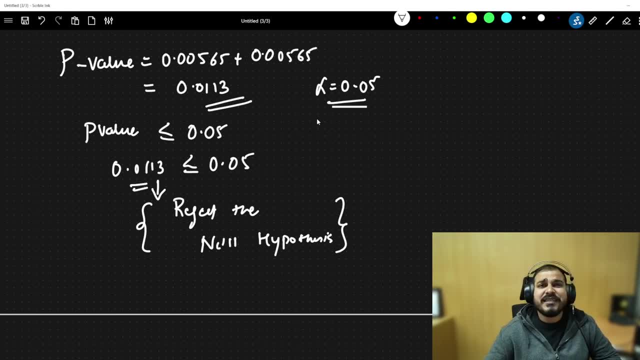 I will solve the problem. This basically indicates that the probability is less than 5%. It's less than. This is the probability Right. This is the probability Which is less than the significance value to support the null hypothesis. So we have to reject it. 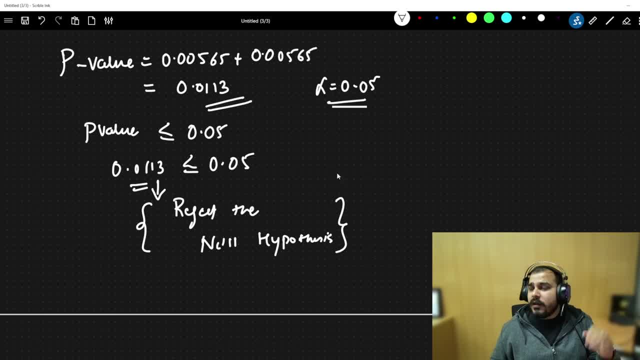 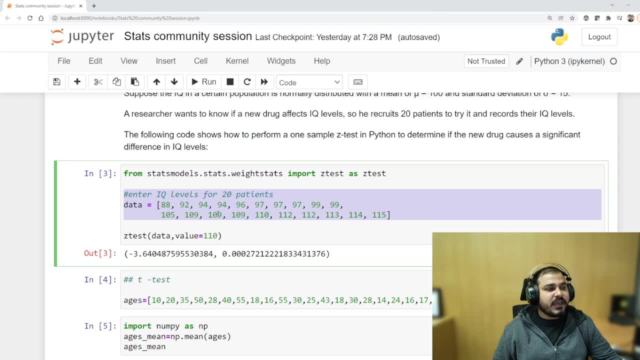 So we are rejecting the null hypothesis, Right? So let me show you one code which I had written in one of my community sessions In day before yesterday community session. Now, in this particular case, let's see, I had the IQ. 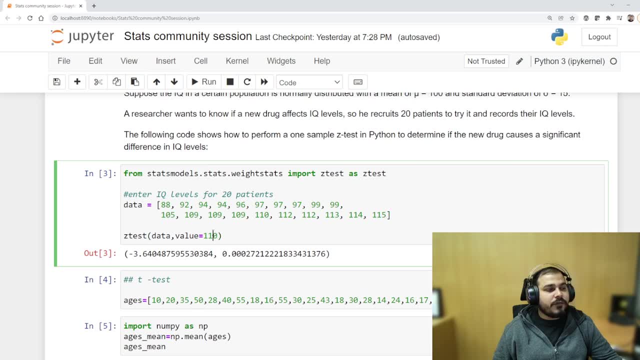 Basically, what I have done is that let's consider that the average IQ of a person, Of a population, is 110.. Okay, And then what I have done? just to test it, I have taken 20 patients, which I can also take more than 30 patients. 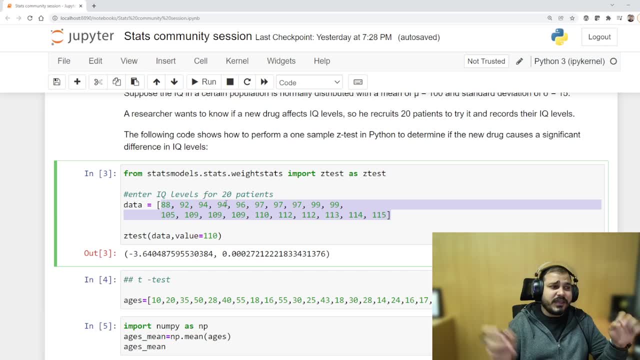 Now don't fight me, Krish. You told Z-test the n-value should be greater than or equal to 30.. I have just shown you one example. You can definitely take 36,, 37, any value. Okay, But understand, I have just taken a sample of values just to test whether it is working fine or not. 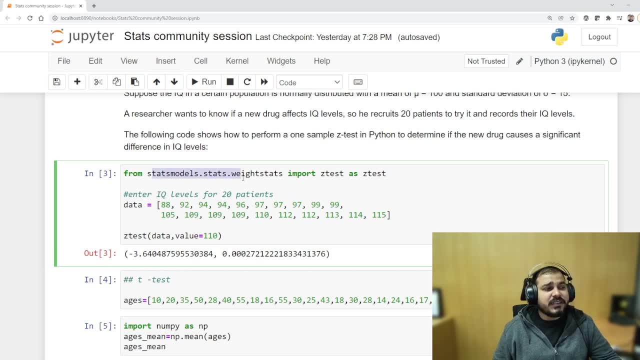 Then, what I have done. I have just used Z-test, which is present in this statmodelsstatswavestats, And here I have given the data And here I am given the population mean. So, once I am comparing with it, I am getting the p-value as 0.0002.. 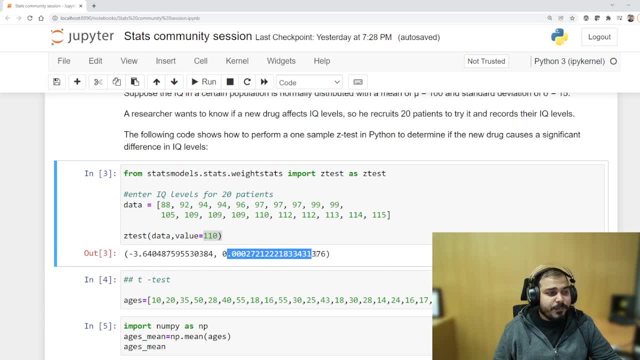 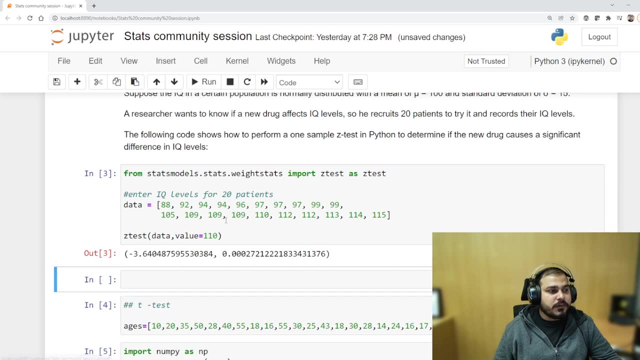 So this is my Z-statistics value And this is my p-value. Okay, Now here I can definitely write a condition saying as if the p-value. See how I will execute it. I will say this: If, if, let me just save this in a variable called as p-value: p underscore value. 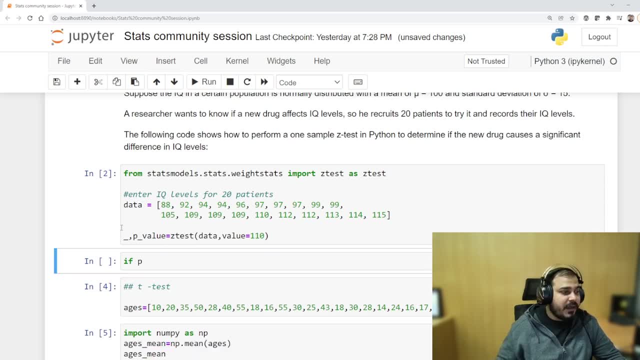 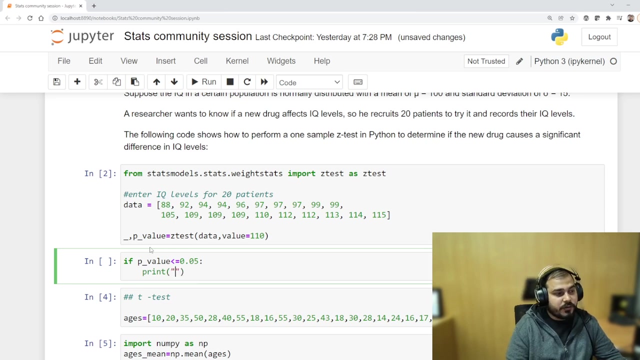 Okay, So p-value. So I will just write a condition saying that if p underscore value is less than, less than or equal to 0.05, then I am going to basically print reject the null hypothesis. So I am just going to write reject the x0..